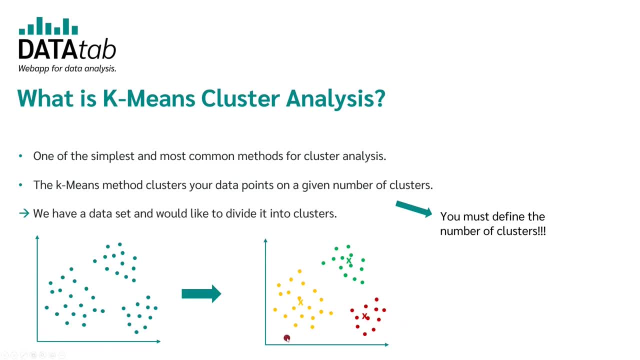 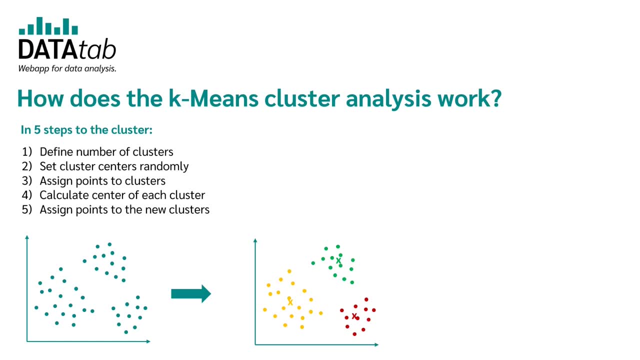 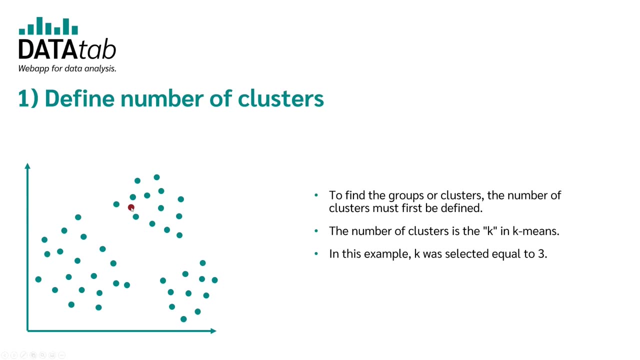 you want to cluster them into three country groups. So now the question is: how does the k-means cluster analysis work? There are five simple steps required. Let's start with the first step. First, you have to define the number of clusters to find the groups or clusters. The number of clusters is the k in k-means. 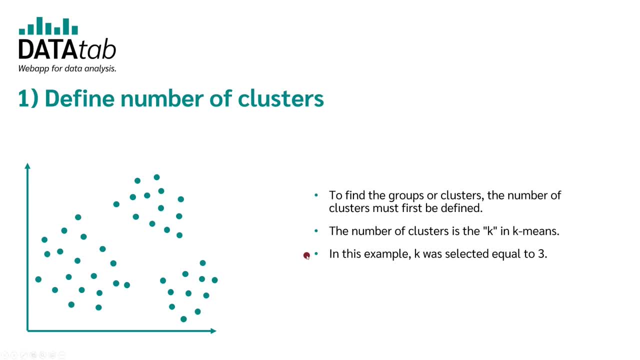 In our case, we simply select three clusters. so in this example, k was selected, equal to three. The second step now is to set the cluster centers random. Each of the centuries now represents one cluster. Let's come to step three Now. we have selected the number of clusters and we set the cluster centers randomly. Now 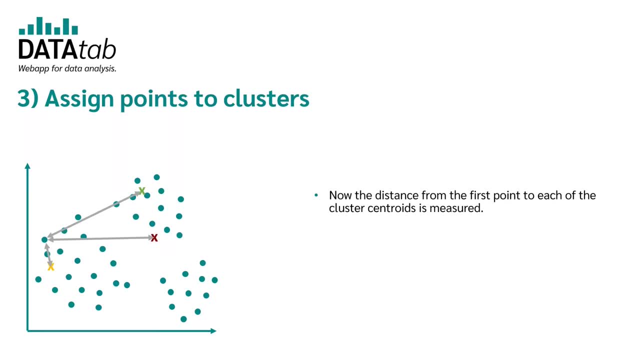 we assign each element to one cluster. So, for example, we assign each country to one cluster. Let's start with one element, And now the distance from the first element to each of the cluster centroids is calculated. So, for example, we calculate the distance from this element to each cluster centroid. 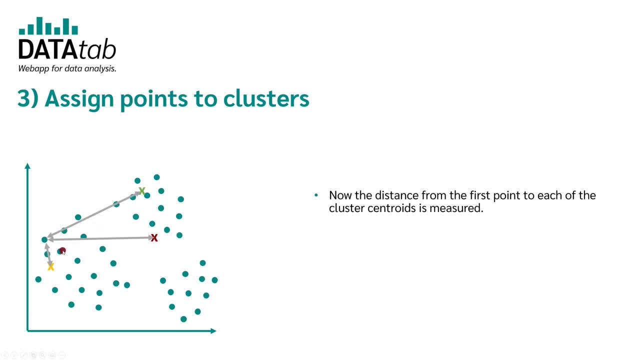 Afterwards, each element is assigned to the cluster to which it has the smallest distance. In our example, the distance between this element and the cluster centroid is the smallest, So we will assign this element to the yellow cluster. Now this step is repeated for all further elements. 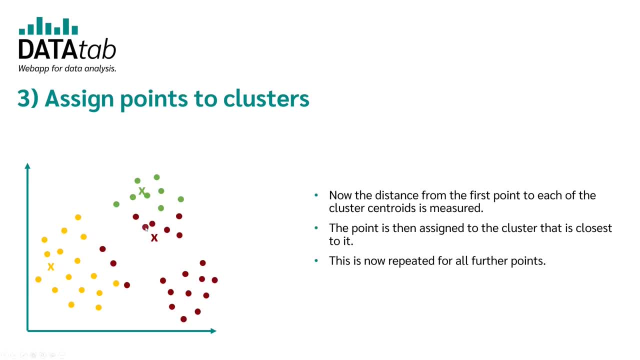 So at the end we have one yellow cluster, one red cluster and one green cluster, And then all points are initially assigned to a cluster. So let's summarize it again: We first have defined the number of clusters. We have then assigned the cluster centroid randomly, and we have assigned each element. 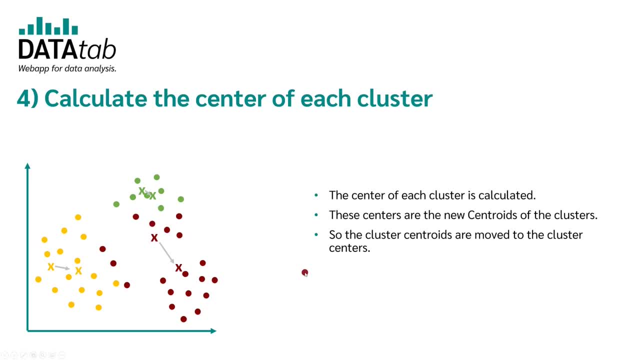 In step 4, we now calculate the center of each cluster. So for the green elements, for the yellow elements and for the red elements, the center of each cluster is calculated. These centers are the new cluster centroids. now This means that we simply shift the centroids into the cluster center. so the cluster centroids. 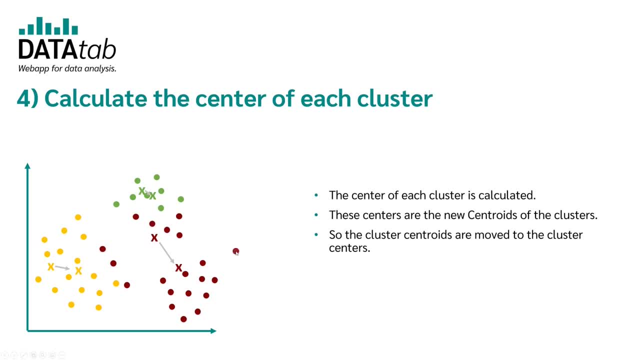 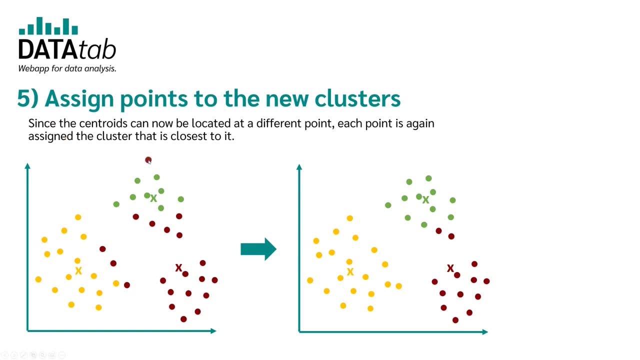 are moved to the cluster centers. now In step number 5, we assign the elements to the new clusters. since the centroids now can be located at a different element, Each element is assigned to the cluster that is closest to it. Now we have finished all steps and from now on step 4 and 5 are repeated until the cluster 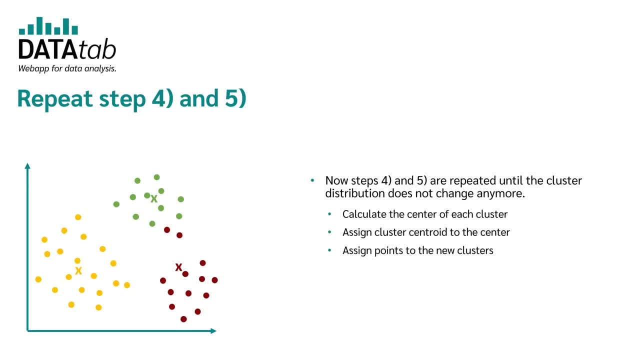 solution does not change anymore. Then the cluster repeats. The cluster repeats. The clustering procedure is over. One disadvantage of the k-means method is that the final result depends very much on which initial clusters we used. To take this into account, the whole procedure is carried out several times and different. 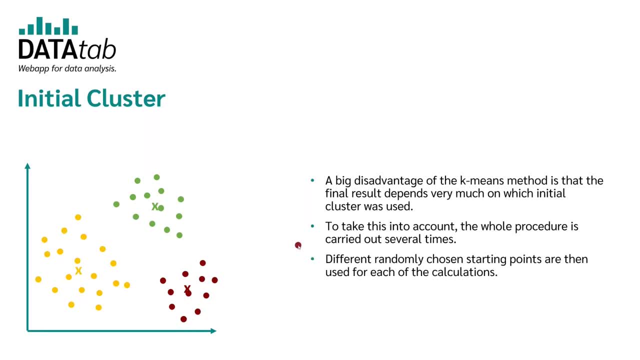 randomly chosen starting points are used for each of the calculations. Each time we use different starting points, it could be that the outcome is different, So we do the whole cluster analysis several times in order to get the best possible result. If you use DataTab to calculate the cluster analysis, the analysis is, for example, done: 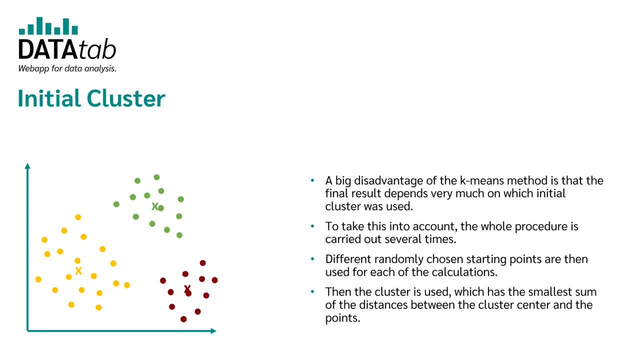 10 times with 10 different, randomly chosen starting points, And then at the end, the best cluster solution is chosen. So the next question is: what is the optimal cluster number? The answer to this question is: what is the optimal cluster number? 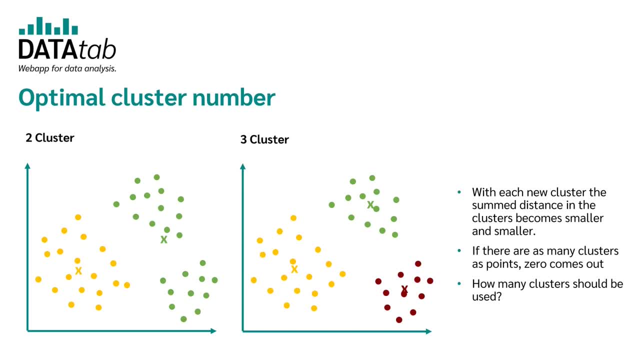 The answer to this question is: what is the optimal cluster number? Each new cluster, the summed distance in the clusters gets smaller and smaller. So if we have a look at this picture where we have 2 clusters and that picture where we have 3 clusters, 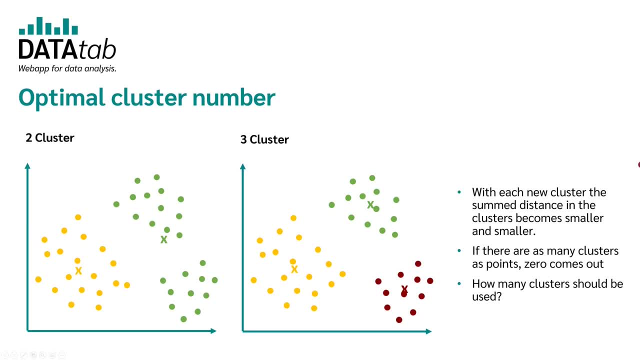 For sure. these 3 clusters fit the data better than these 2 clusters. The distance between the elements and the clusters is in this case, higher than in that case. So the question now is how many clusters should be used? answer this question: we use the elbow method. With each additional cluster, the summed distance 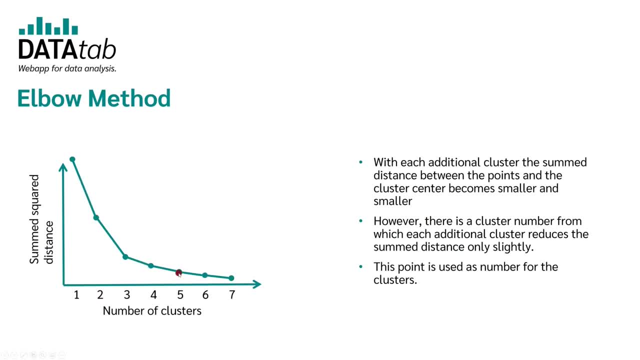 between the elements and the cluster center becomes smaller and smaller. However, there is a cluster number from which each additional cluster reduces the summed distance only slightly. This point is used as the number of clusters. So if we have a look at this plot, we can see that 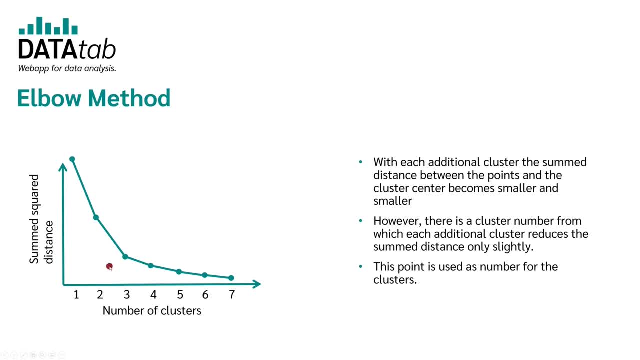 there is a big gap between cluster number one and two, And there's also a big gap between the number of clusters two and three, But there's only a small gap between number of clusters three and four. So in this case we select a number of clusters, of three clusters. Now I'd like to show you. 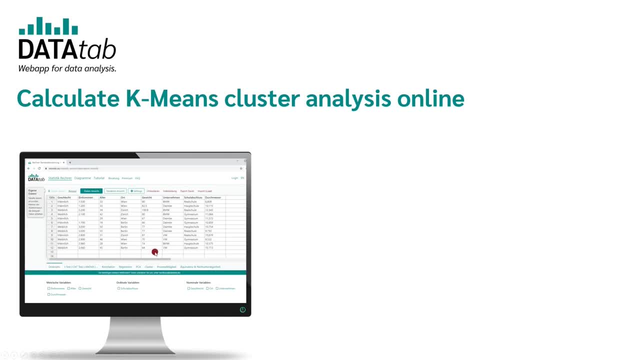 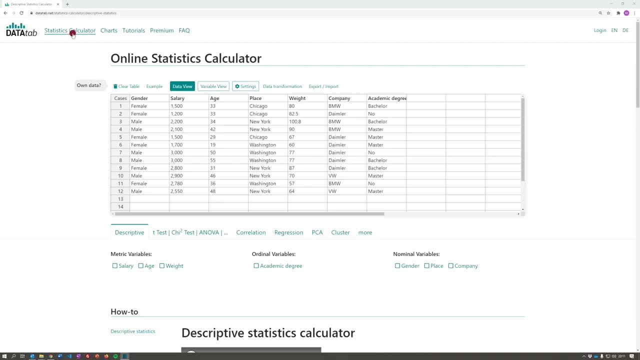 how you can easily calculate a k-means cluster analysis online with DataTab. To do this, please visit datatabcom And click on the statistics calculator. In order to calculate a cluster analysis, you simply choose the tab cluster. If you want to use your own data, you can clear the table. 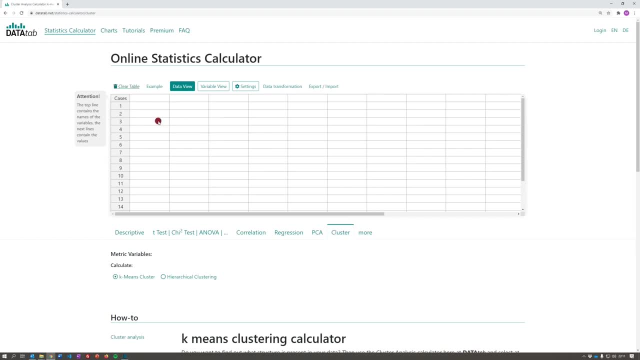 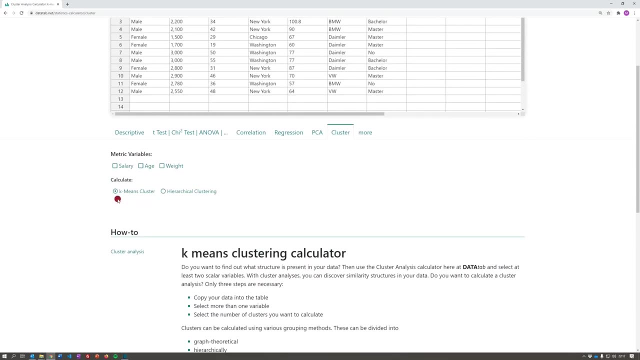 and then copy your own data into this table. I will simply use the example data now. So I want to calculate a k-means cluster analysis. Let's say we want to cluster a group of people by salary and age. First we need to calculate the number of people by salary and age. 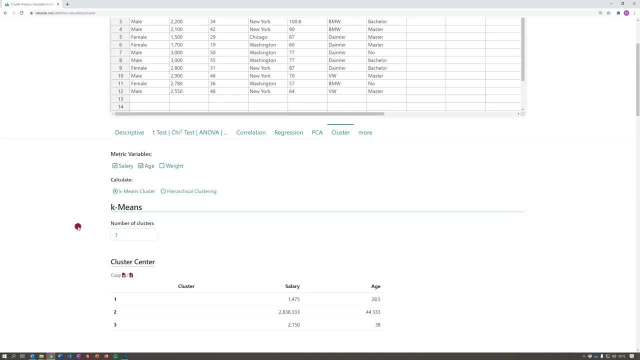 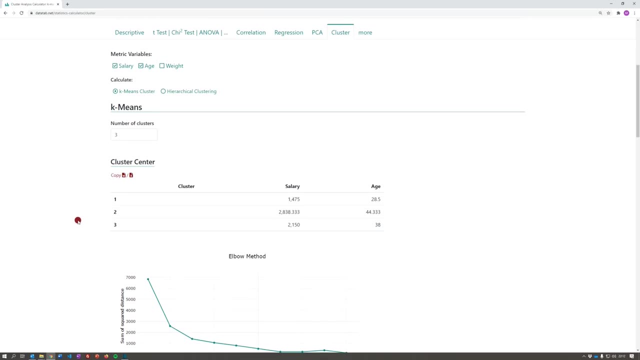 First we can define the number of clusters, and we enter the number of clusters, DataTab will now calculate everything for you and you get your results right away. So here you can see the three clusters with the centroids, and there you can see the elbow method. 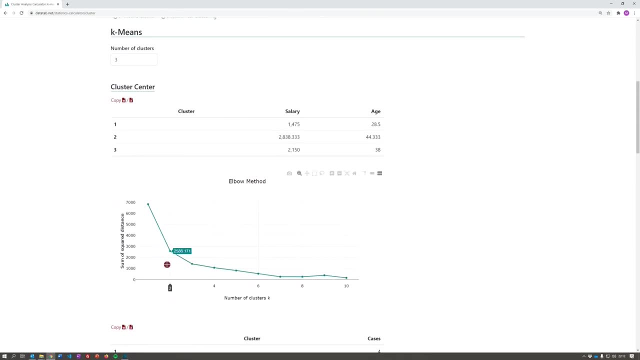 In this case, the results indicate that we should use a solution with two clusters. We have selected three clusters before, so we can change it in order to get the best suitable number of clusters. But let's go through the results now step by step. Here we can see how 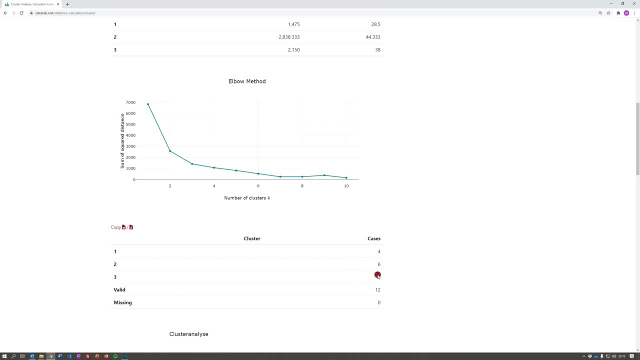 many elements are assigned to the different clusters, And here we get the plot with the different clusters. Here we can see one cluster, we see one cluster there and we see another cluster here. Further we get a table where each element is allocated to a cluster. If we now choose two, 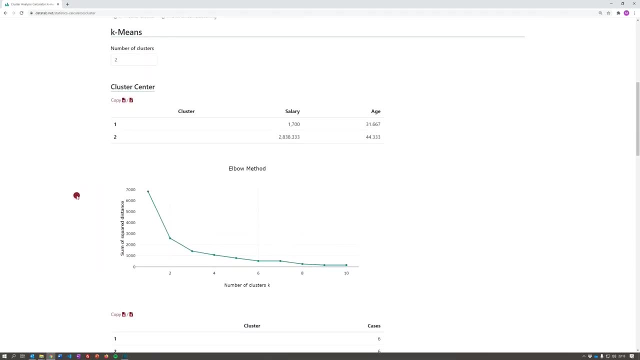 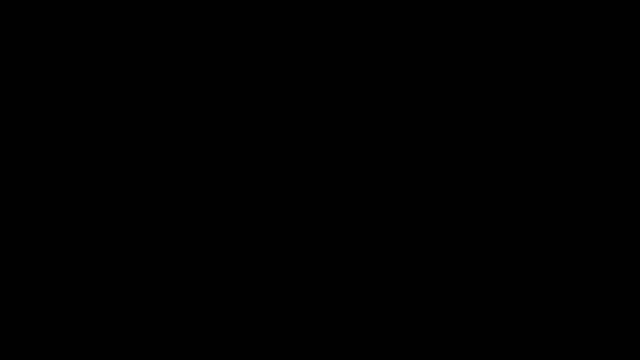 as the number of clusters, we get new results If we now choose two as the number of clusters, and we can see them here. In this plot, we have one cluster here and one cluster there. Moreover, we can see that the two clusters fit the data quite well. Thank you for listening.